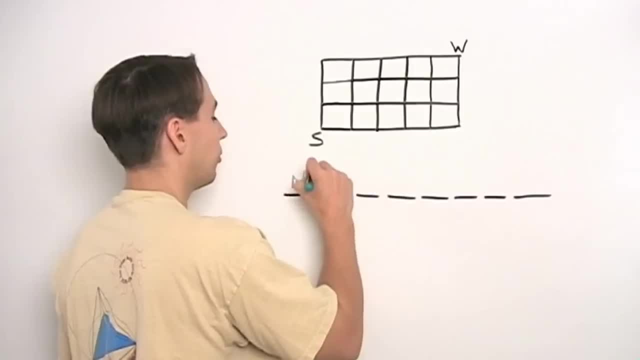 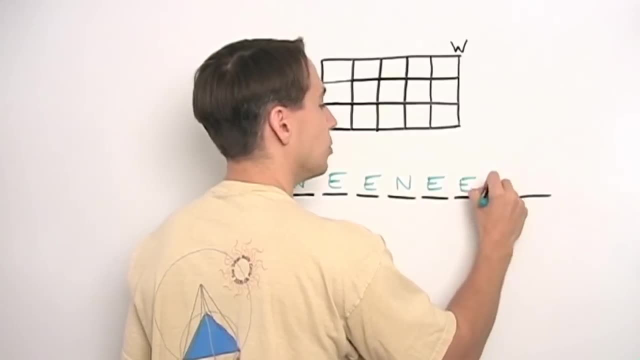 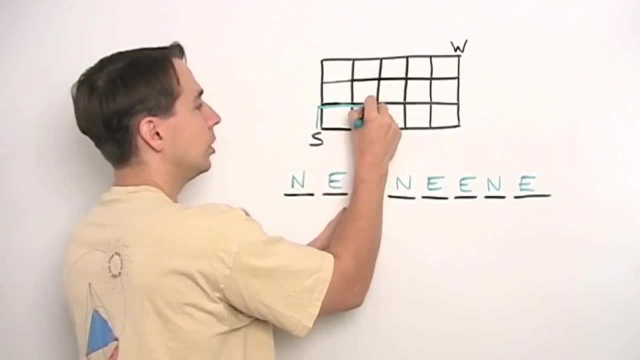 For example. here's one route I might take. I might go north, first east, a couple times north, again east, a couple times more north and then east. So I'm going to draw that up here: North to east, One more north. 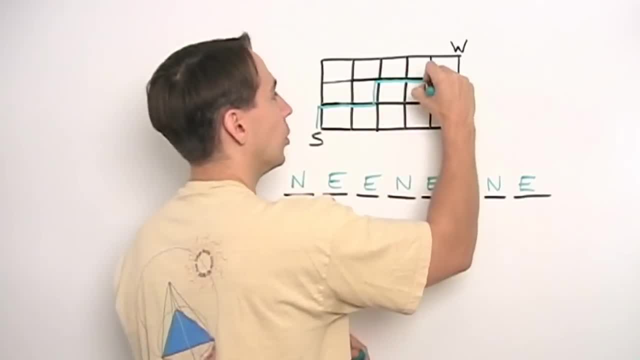 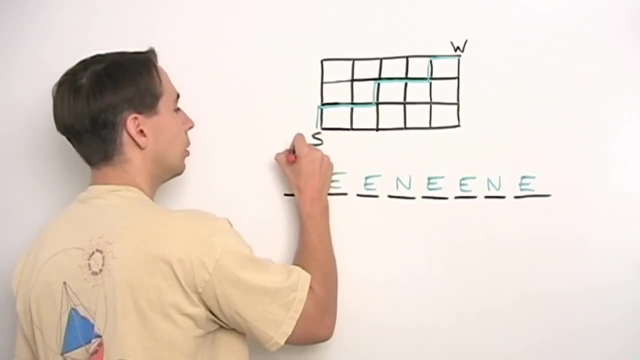 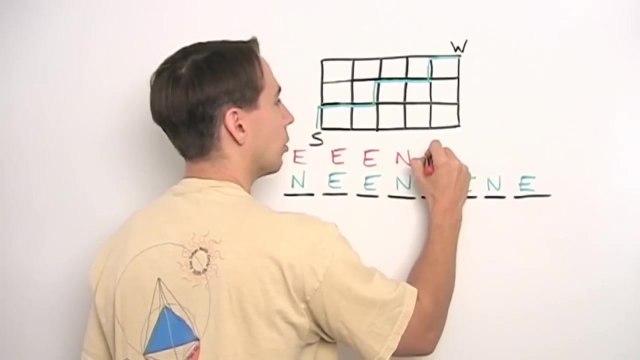 A couple more east, One more north and then east into work. So there's one And here's another one. Draw this one in red. I'm going to start off going three east, one north, a couple more east and then a couple more north. 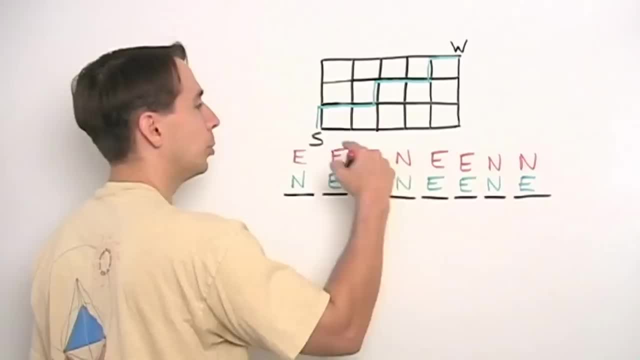 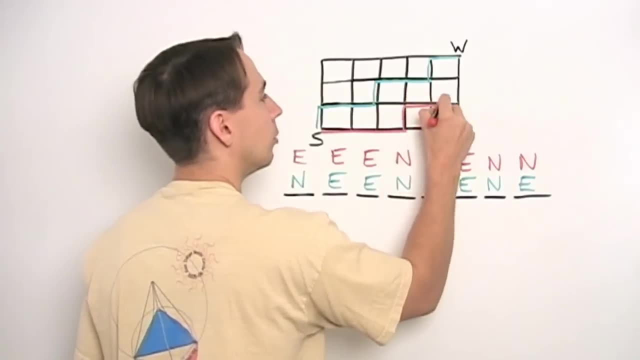 So I know I need three norths and five easts, so I'll be putting three N's and five E's in here. Let's go ahead and draw that. one. Three blocks east, One north, Two east, Two north. So those are two of the paths. 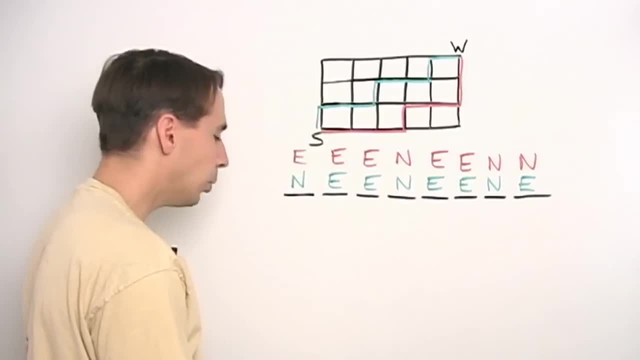 Now, looking at this, I could figure out. hey, now I can see how to count them. I know I have to take eight steps. I'm going to have to take eight steps Now. I'm going to have to pick three of them to be north. 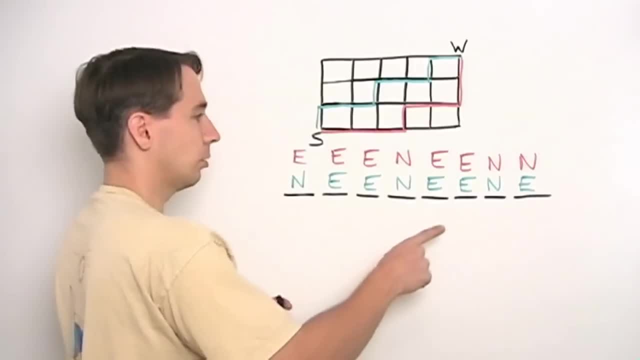 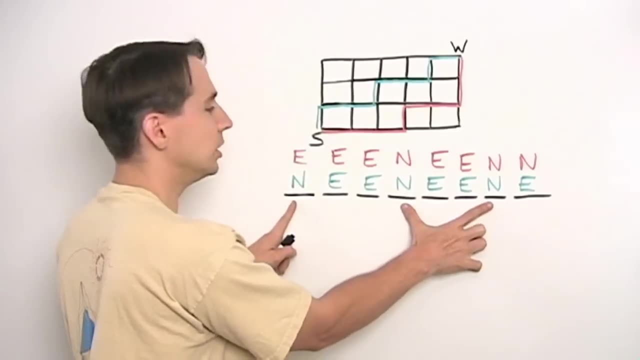 Now, at first I might think that's eight times seven times six, Because I could pick this one to be north and this one to be north and this one to be north. But then I realized, wait a second, It doesn't matter what order I choose these three to be north in these. 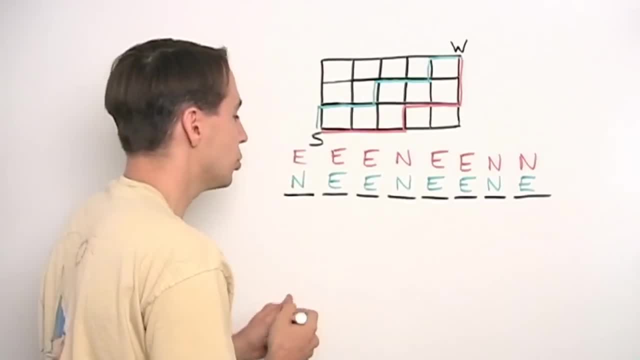 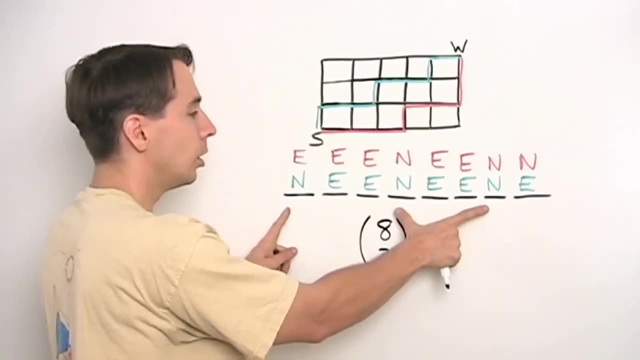 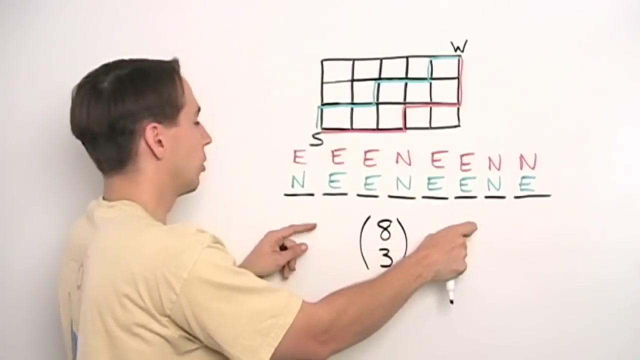 So what I really have here is a combination. I want 8. choose 3 ways to do this, because if I'm going to pick these 3 to be North, it doesn't matter what order I pick those 3.. I can pick this one, then this one, then this one, Or I could have chosen this one to be North first, then this one, then this one, So the order doesn't matter. 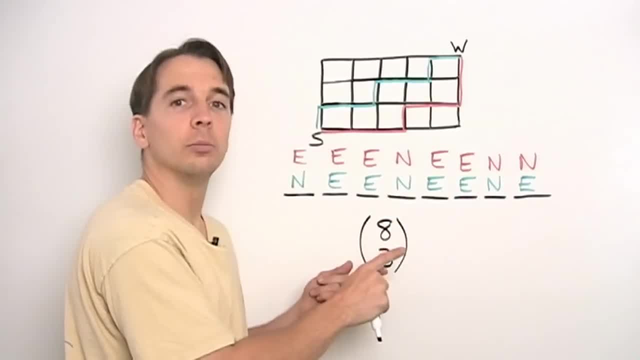 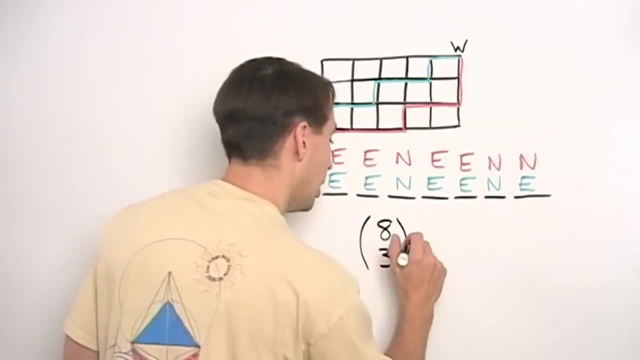 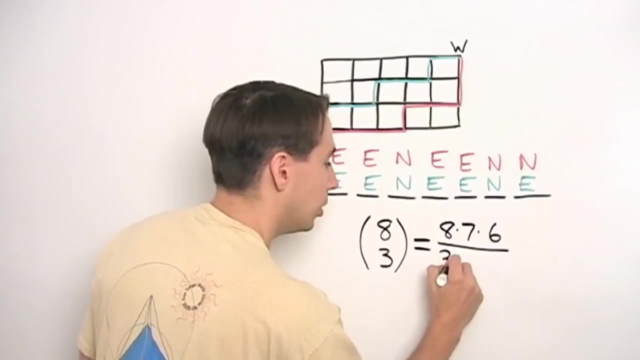 I have 8 slots here. I have to choose 3 of them to be North. So there are 8. choose 3 ways for me to pick 3 of my 8 steps to be North And I know how to compute that. That's pretty easy. 8 times 7 times 6 over the 3 factorial for the 3.. 3 times 2 times 1.. 3 and 2 makes 6.. 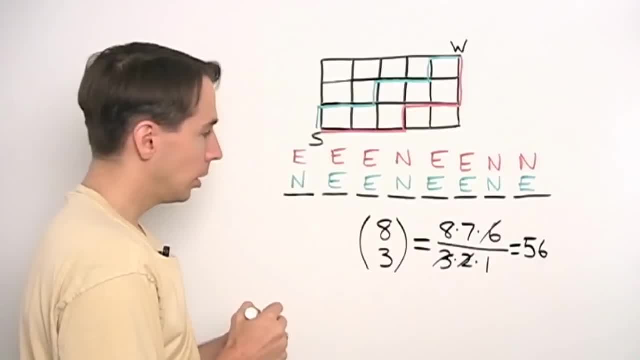 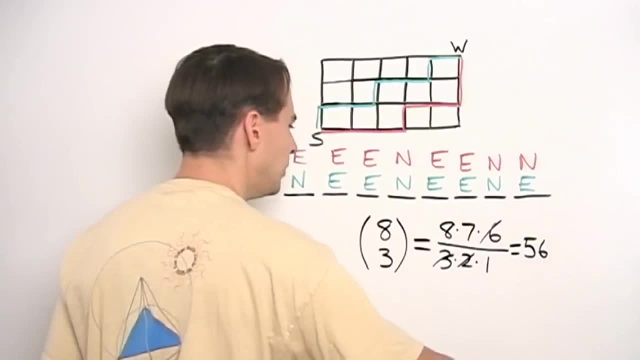 56 ways for me to get to work. But you know, some days I'd be going in and I'd know I'd know I have a rough day ahead. Those days I might want to take a little extra time to get to work. 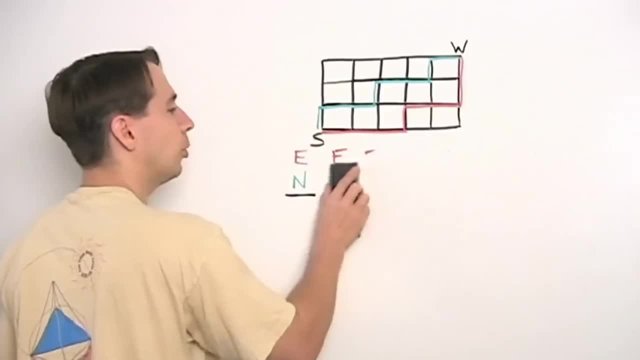 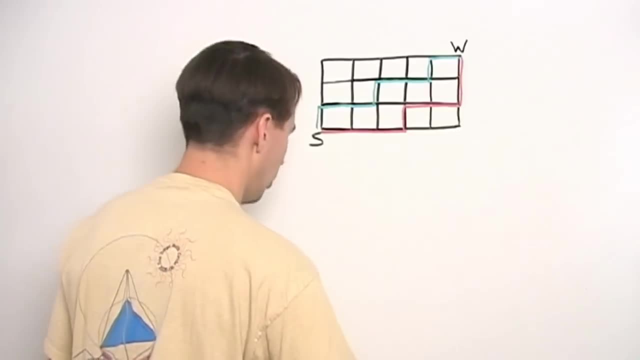 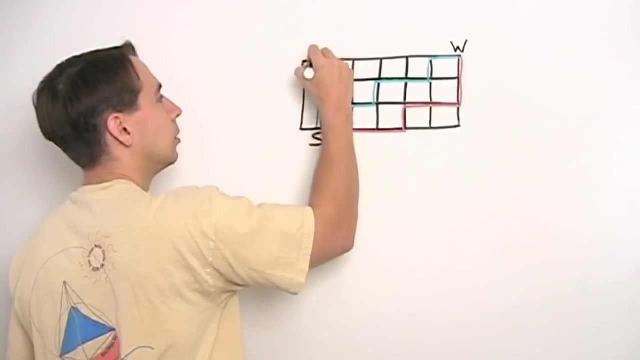 So I'd mix things up a little bit and I'd throw in one step to the West in my route So I might come out of the subway and go West immediately. So basically I add it on Or I might add one on out here. 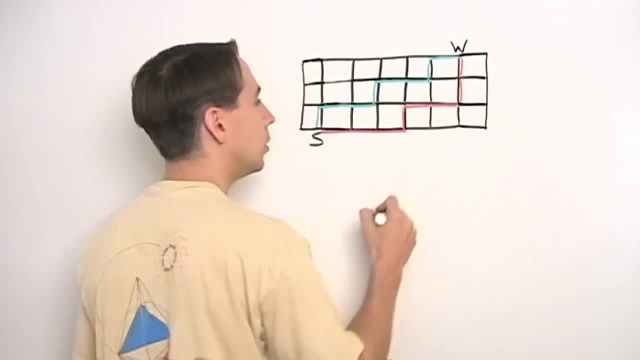 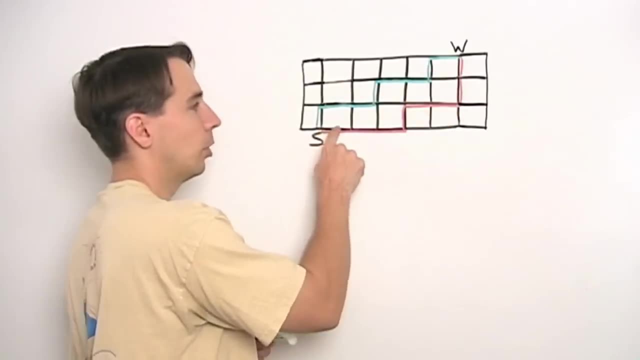 Or I might add it on in between. You know I go over up, back one up, and then on to work, Or I might come all the way over here, go up back to work, Hmm, So if I want to change these paths, you know, maybe I erase this. 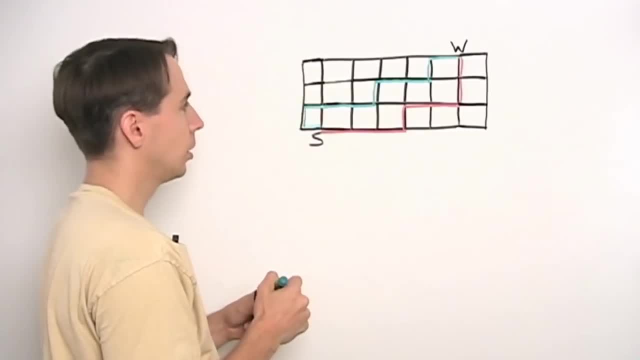 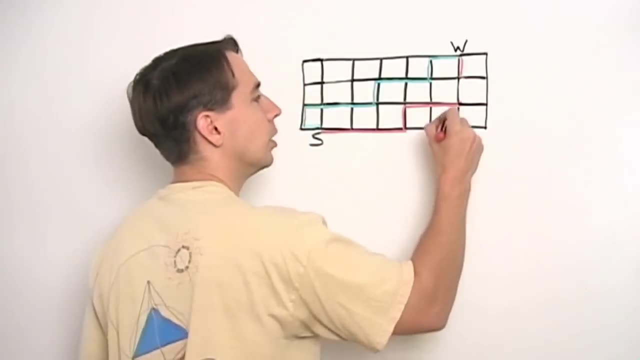 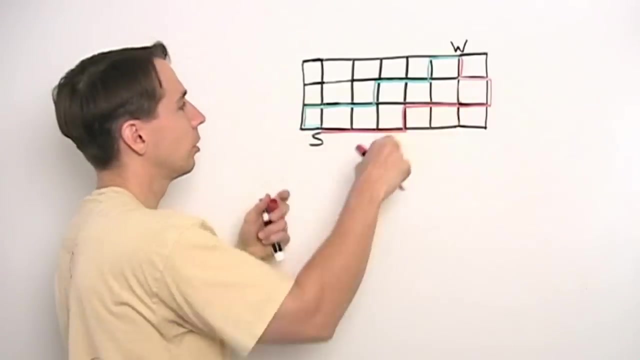 And I go West first, then up, then over, And let's see what might we have done here. Instead of that, we go out up and back. So you see, each of these has one step West in them. Now, if we're going to take one step West, that means we need to throw in an extra step East too. 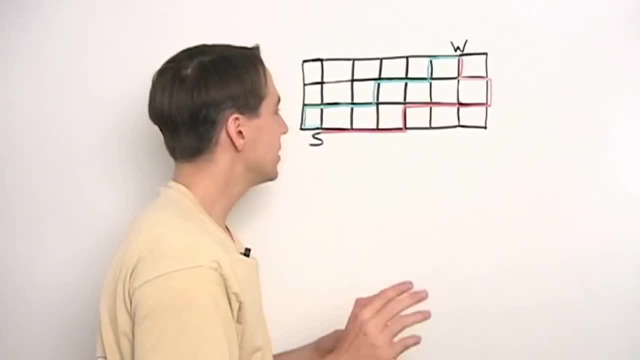 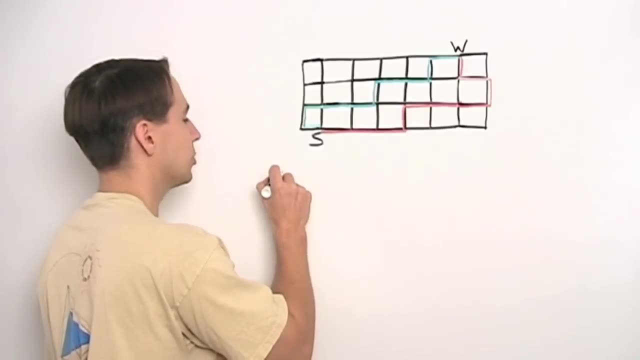 To make up for that one step West. So now I know I'm taking a ten-step path. So when I'm riding the subway and I sit there and I need to lay out ten steps as my plan. So let's see: one, two, three, four, five, six, seven, eight. 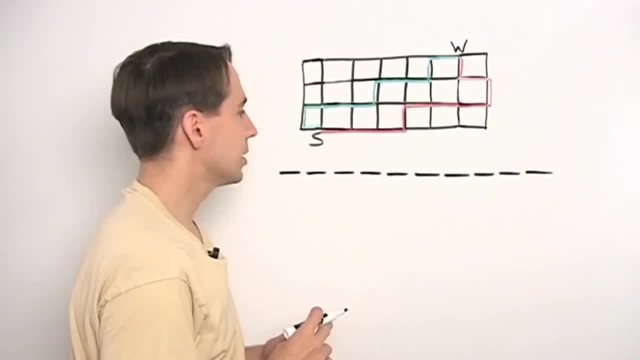 Ten, And of course we're going to count how many different paths I can take. So the first thing I would do I'd look at that and be okay, I've got ten choices, I'm going to choose the West step first. 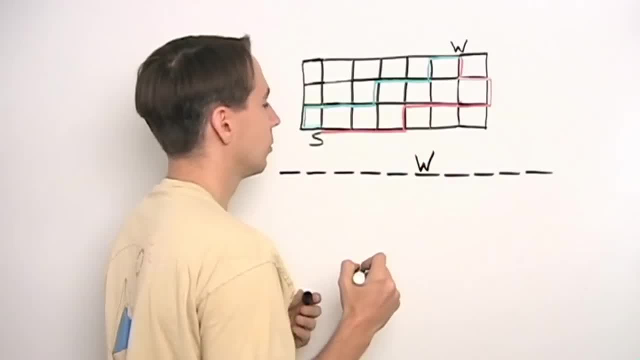 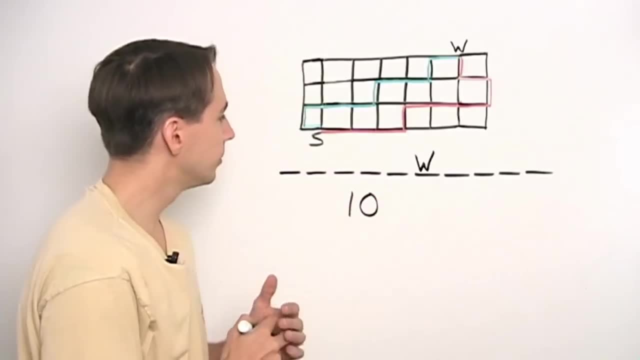 Oh, let's see, I'm going to pick, say I pick this one, And there are ten ways I can do that. So ten ways to choose the West step. So we start with our ten. Now what? Well, I have nine steps left. 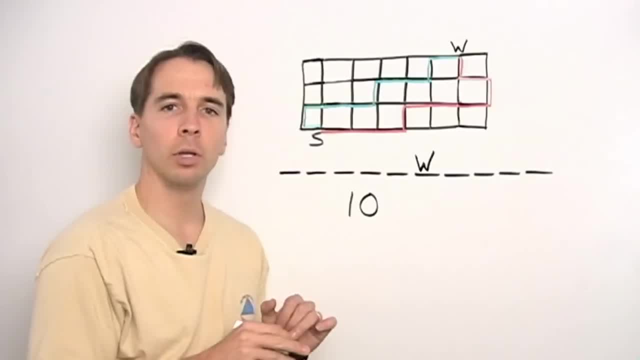 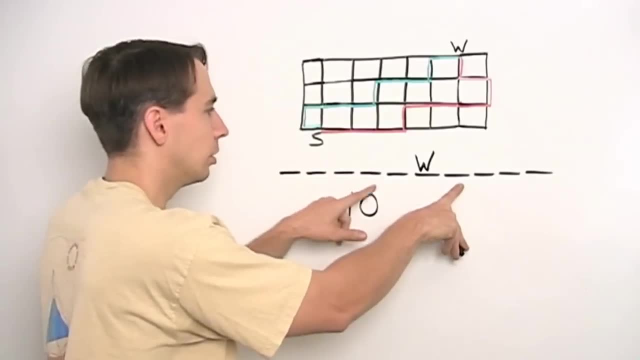 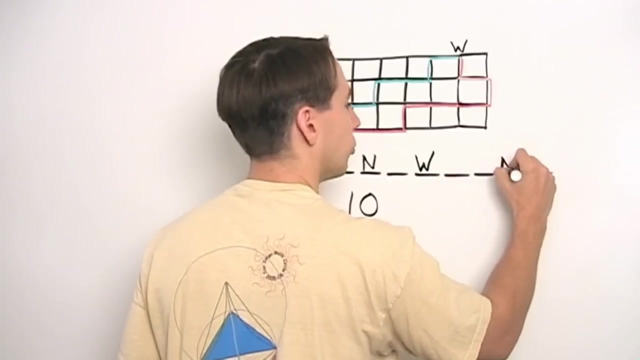 And I have to choose three of them to be North. And, just as before, it doesn't matter what order I choose three of these blanks to be North, I just have to choose three different ones. You know, say I choose this one, this one and this one. 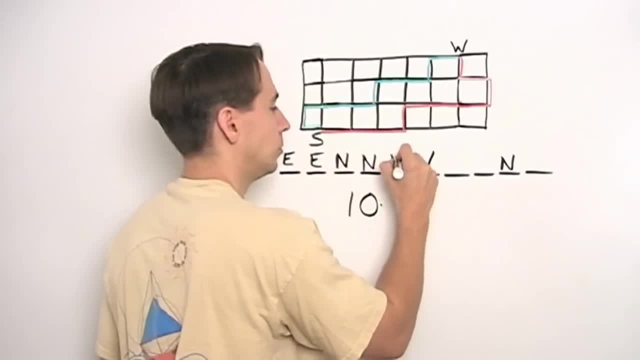 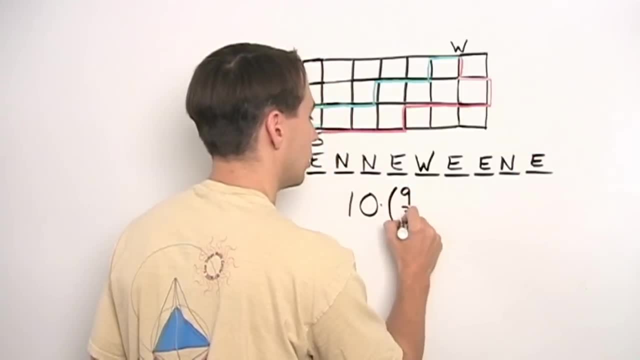 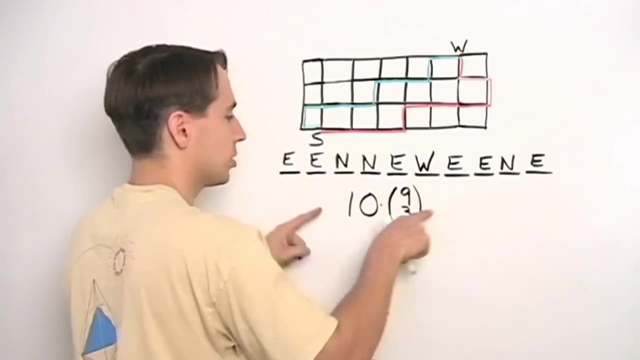 Then the rest have to be East. So I see that of those nine blanks I had left, I have to choose three To be North. So for any place that I choose, the West. so for any of these ten choices where we're going to put that step West, 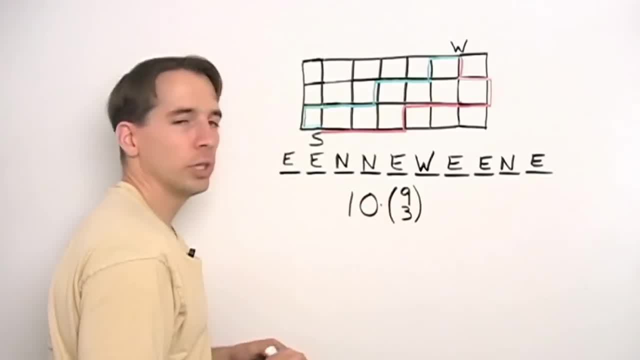 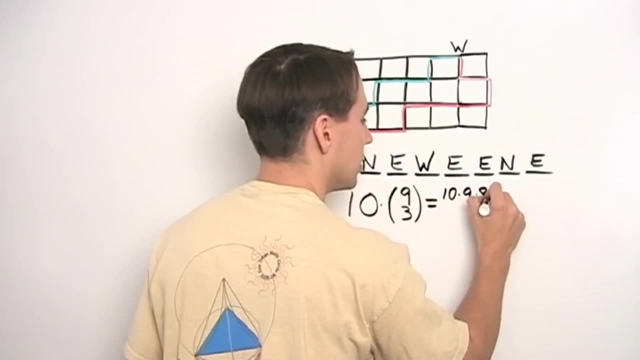 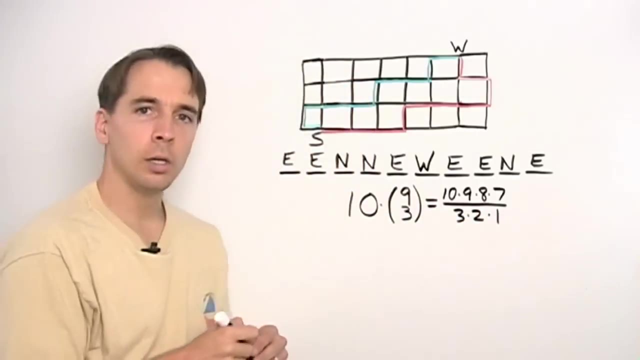 I'm going to have nine, choose three ways to put in the ends, And then all the rest are just Es. So now I can just figure this out: Ten times nine times eight times seven, Divided by three times two times one. And before we compute this you might think: well, can we check our answer here? 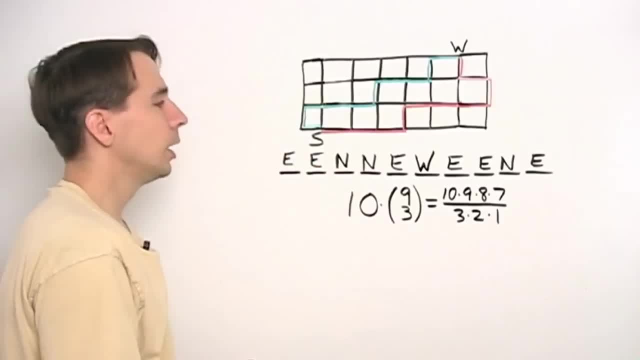 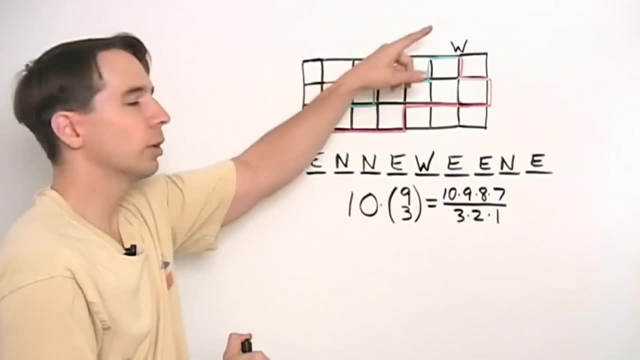 Is there a number? Is there another way to do this problem? And we see eenie weenie up here And we think, hey, we can use eenie weenie Because no matter how we order these letters, that gives us one of these paths. 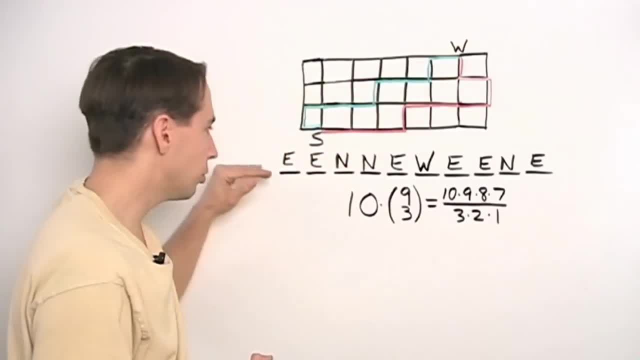 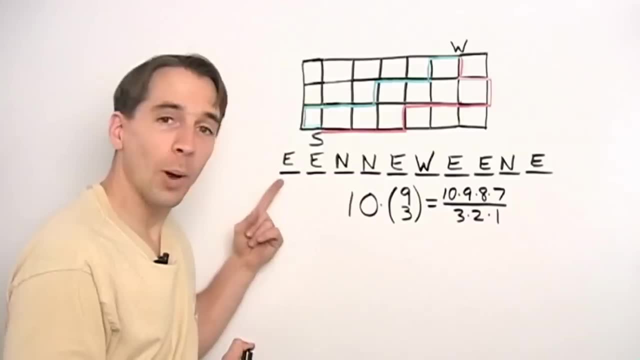 So, really, in order to count the number of paths we have here, all we're doing is counting the number of different words we can make when we rearrange the letters in eenie, weenie, And we know how to do this problem already. 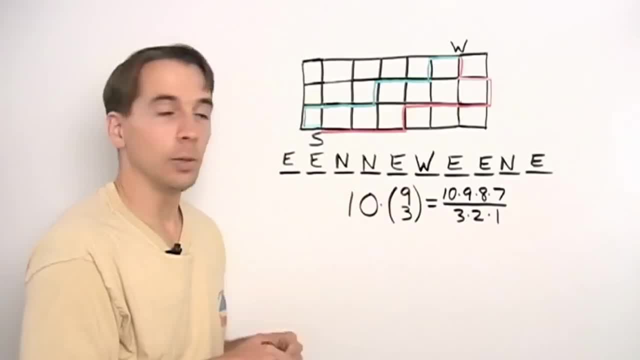 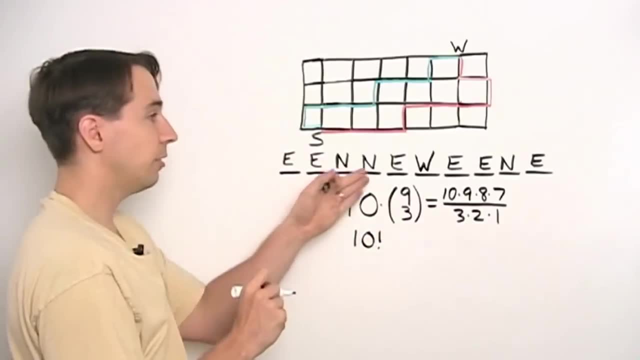 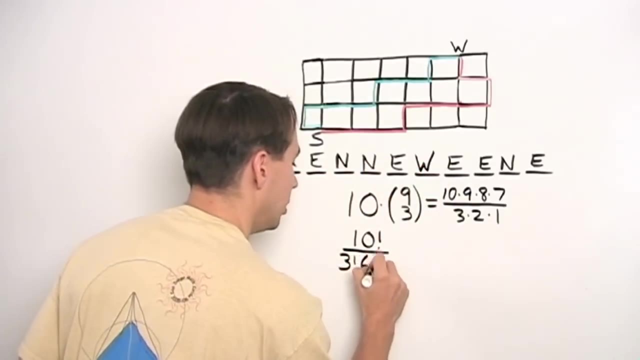 We know how to count the number of ways we can order the letters in eenie weenie. There are ten letters in eenie weenie And then we have to divide by three, factorial for the ends, And then we have to divide by six factorial for the Es. 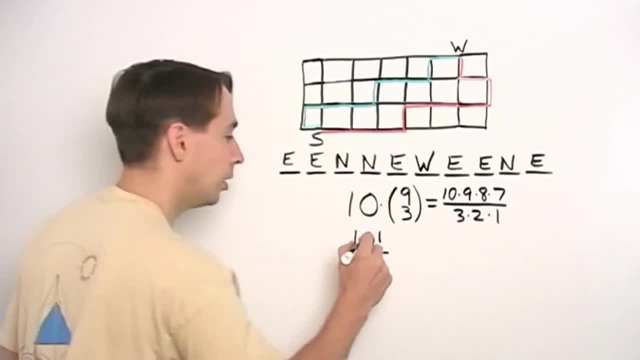 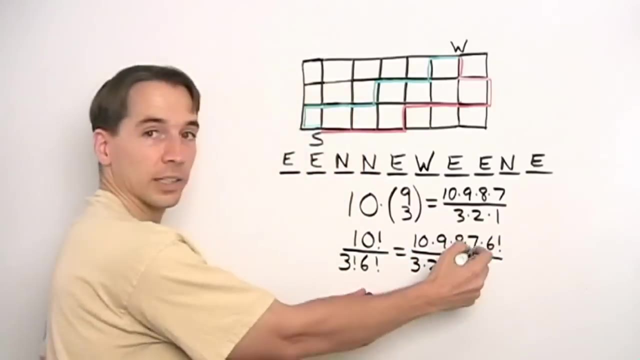 Now, at first you might think, wait a second. these answers look different. But when we write ten factorial as ten times nine times eight times seven times six factorial, we see our answers are the same Because the six factorials here they cancel. 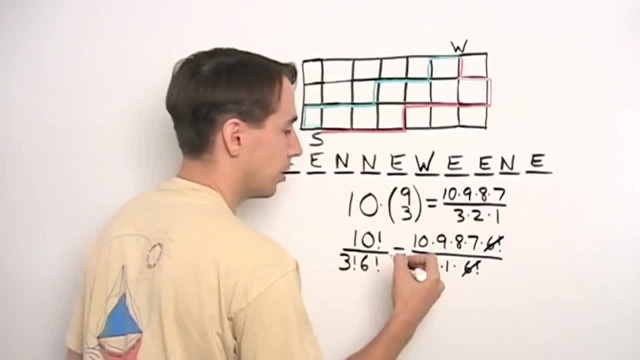 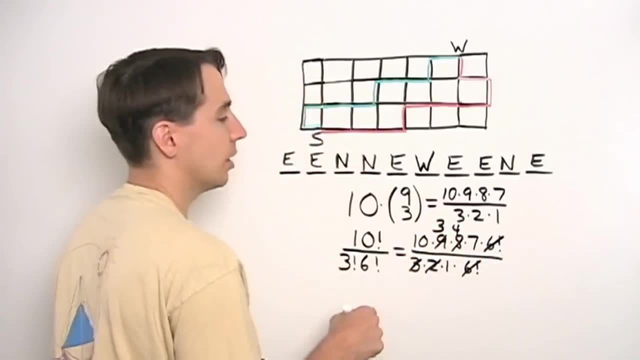 And these two numbers are the same, And then we can just sit there and we can do the arithmetic. now: Three cancels with nine leaves three. Two cancels with eight leaves four. Three times four is twelve times seven, That's eighty-four times ten is eight hundred and forty. 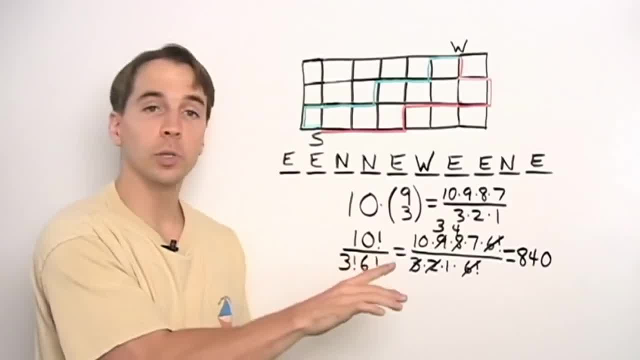 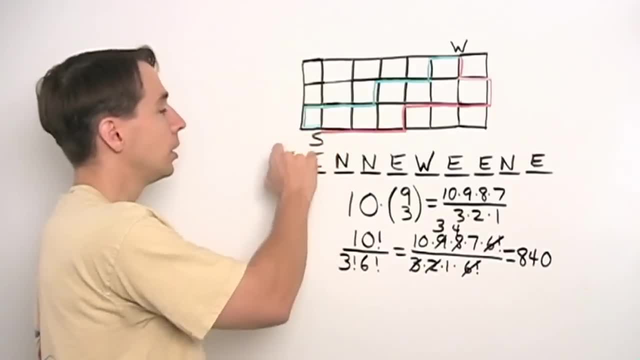 So we see that we have eight hundred and forty ways. Once we just throw in that one west, it makes us choose the extra east as well. Now we have eight hundred and forty ways To get from the subway all the way up to work.